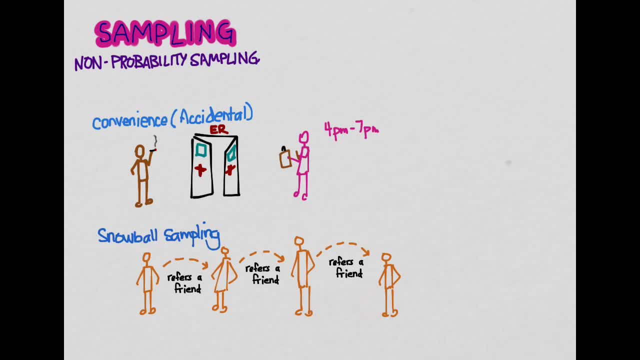 Among all of them. that could be a confounding variable as well. So this is not a good sample either. In purposive sampling, sometimes also called judgment, this is a fundamental sampling. The researcher depicted here with a magnifying glass because he's trying to research something. 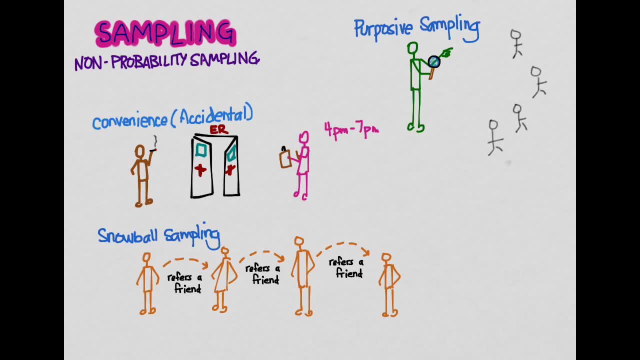 this person picks who is in the sample, So they try to use their own judgment. So they might say: you know what, we'll pick you, not you we'll pick you and we don't want you, And so this is obviously not random and you can only imagine that it's what the researcher thinks is important. 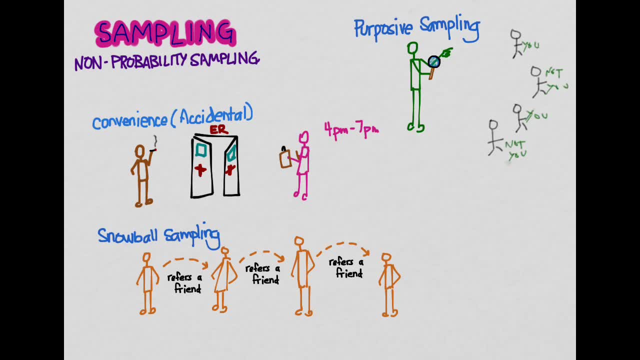 so other confounding variables could easily be used. And yet another kind is called voluntary sampling, in which people volunteer to do the survey, Because in this kind of sampling you have people who have self-selected themselves and so there's usually some reason. It's usually people who are either upset or people who have some other reason that they want to be included. 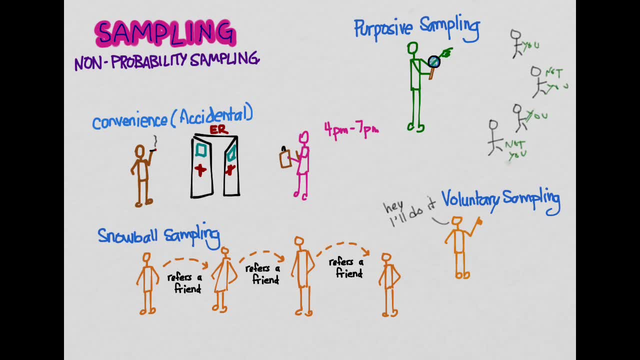 So it's not random. There is something that is making them volunteer to become part of the sample. So what you'll see that is common among all of these non-probability sampling techniques is that there is no randomness involved. Usually it's just people picking because of the time of day, someone telling a friend to join, or the researcher picking on their own. 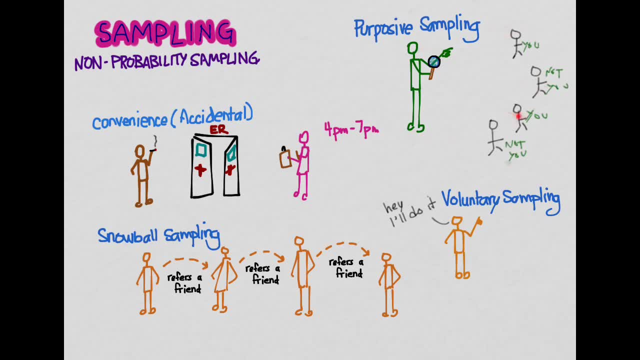 or letting the person pick, And so the samples are not random. And when they're not random, you lose the ability to get rid of confounding variables. variables and spread them out, because there's some. there is something that makes the all these people. 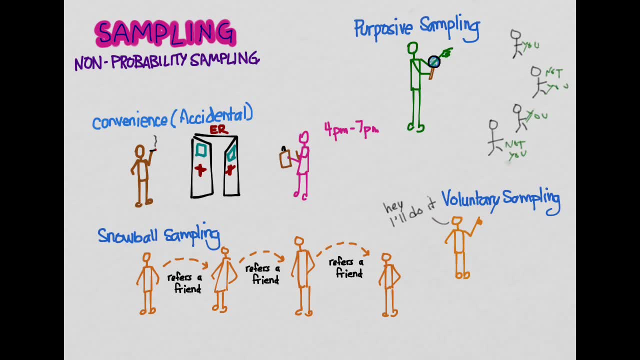 similar right and that it could be. what is the thing that confounds your study? an alternative factor that could explain the cause that you're looking for? so these are different methods of sampling, but first we looked at the probability sampling, which is important for random sampling, and then these are the non probability sampling, and these can lead to bias. you can even have bias. 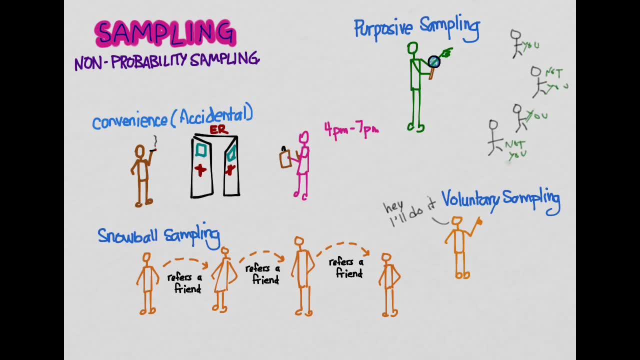 in probability samples as well, but if you're going to use one of these non probability sampling techniques, you're more likely going to get that okay. thanks, bye.